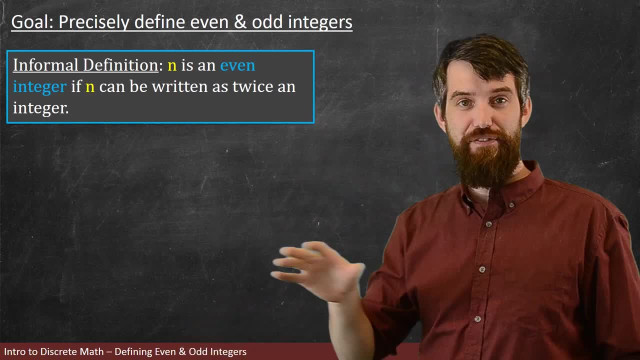 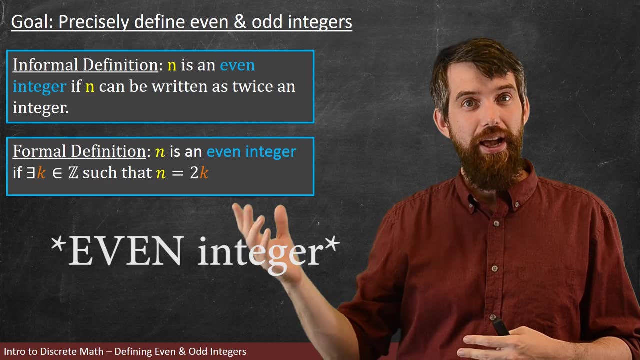 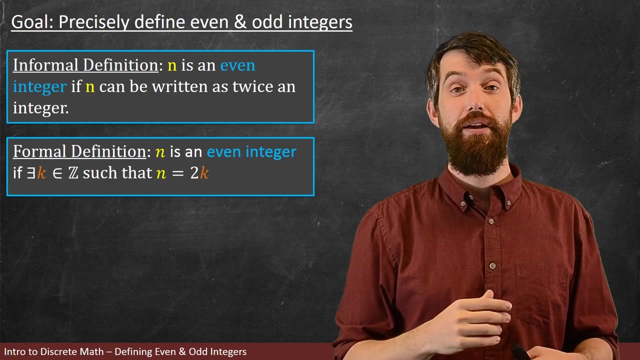 as twice it. So if I want to take this informal definition and make it into a formal one, I might write something like this: I would say that n is an integer if there exists another integer, k. So there exists k in the integers, but has the property that the n is twice k. now why do i like this formal? 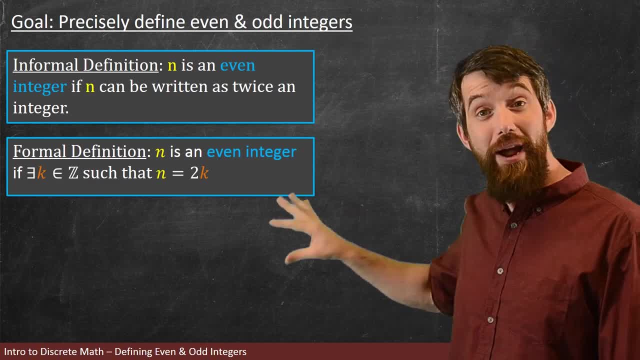 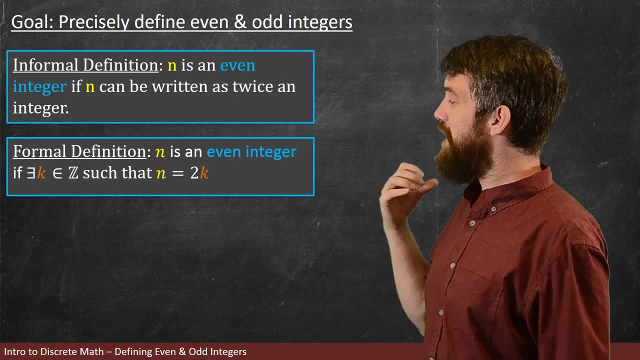 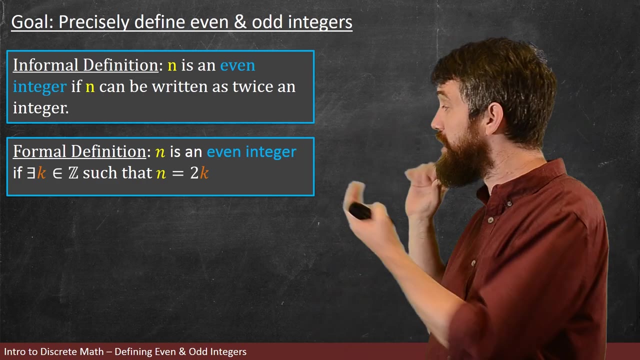 definition. so much it's because now there's actually an equation here: n equals 2 k, and i know something about what k is. k is an integer, so if i want to make a proof that involves the even integers, now i can actually substitute it in. i can write equations. i have a precise way of writing. 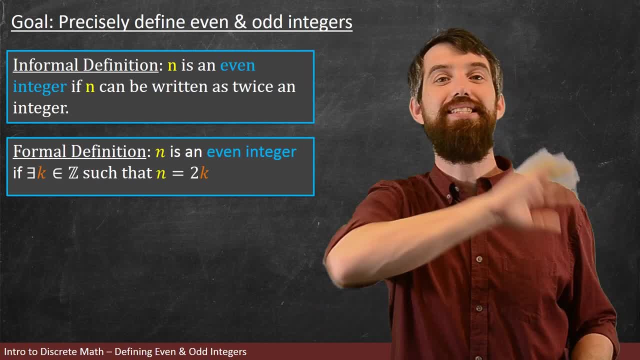 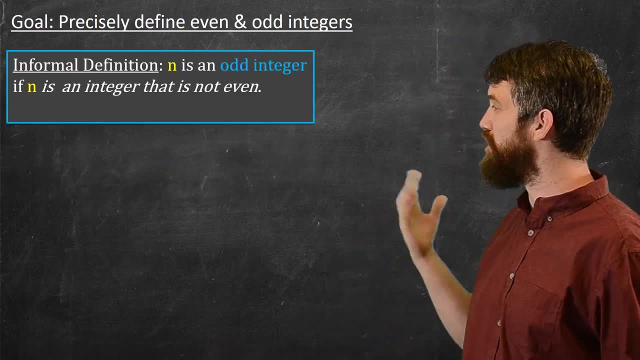 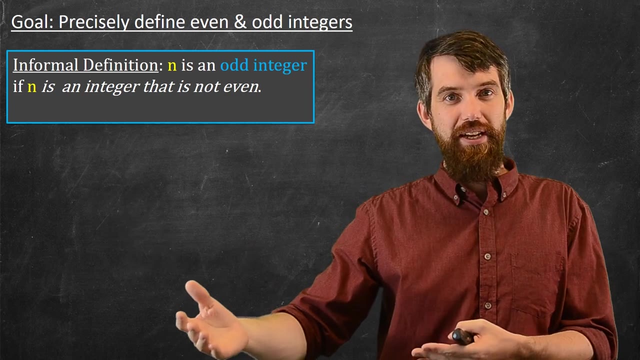 what i mean when i talk about an even integer. okay, same story, but for the odd integers, well okay, what's an odd integer? informally, odd integers are the integers that are just not even. as in: if two, four, six, eight are even integers, then the other ones, the one, three, five, sevens, those are 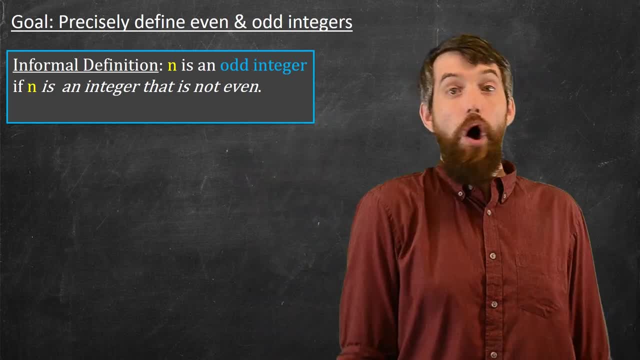 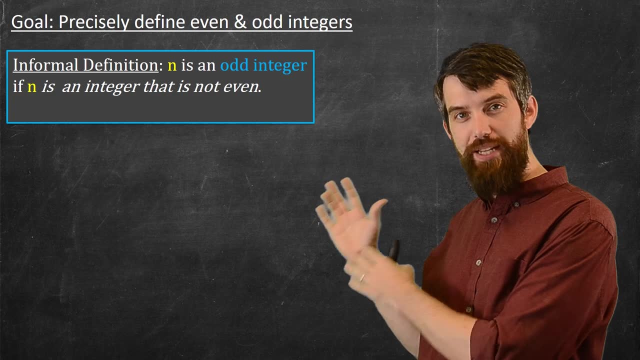 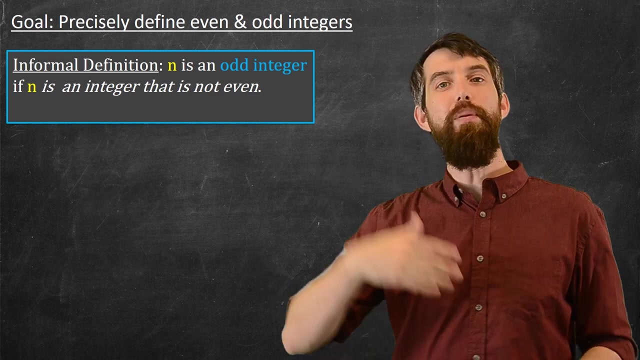 the odd integers. okay, that's not bad. you are allowed to define something as being not some other thing. okay, but let's try to be a little bit more precise about this. if i take, say, six, we said that was even because it was twice an integer. but what about seven? so seven is odd. but what i notice about 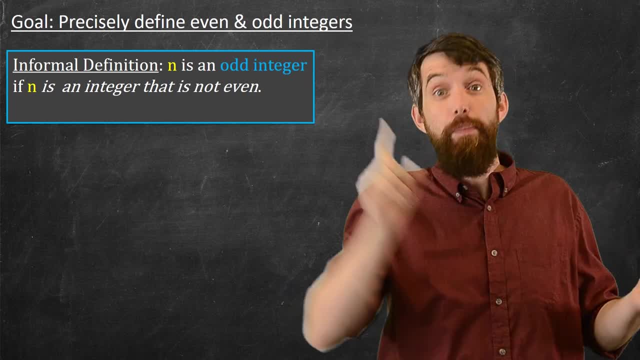 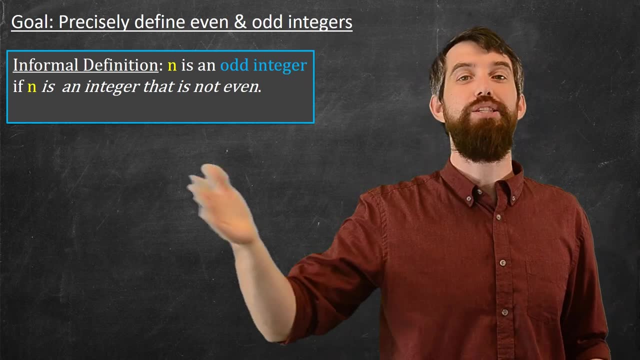 seven is that it's twice an integer, twice three plus one. so all of the odd integers can really be written as twice an integer plus one. so i'm going to use that as my formal definition. again, it's an existential claim. i'm saying there exists a k. 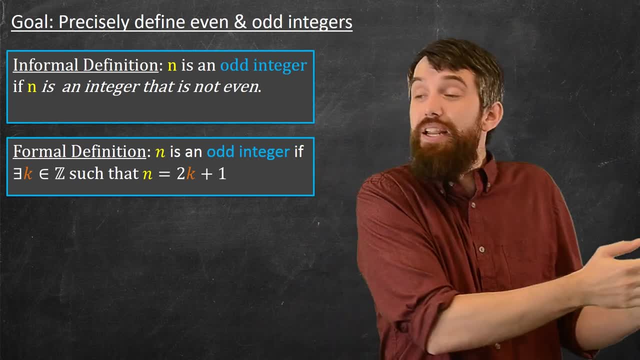 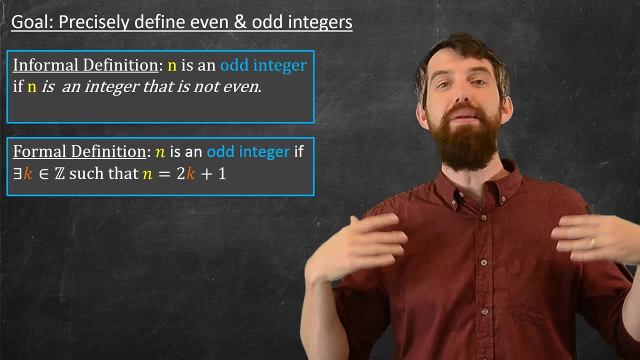 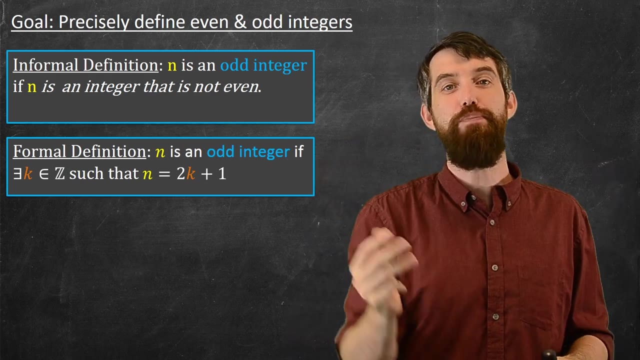 the integers such that your odd integer n can be written as twice k plus one. and now again i have a precise formal definition of what i mean by odd integers. there's an equation here. i can substitute that equation into other equations and i can use these definitions to make proofs about the even. 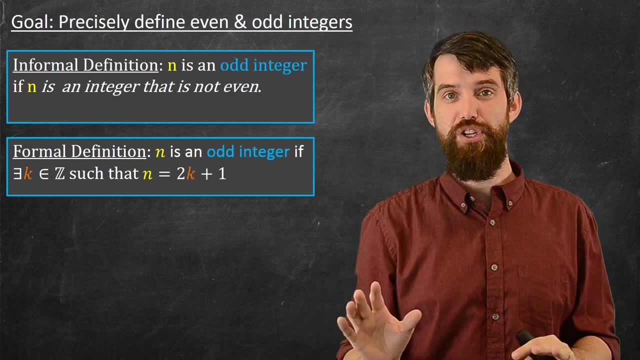 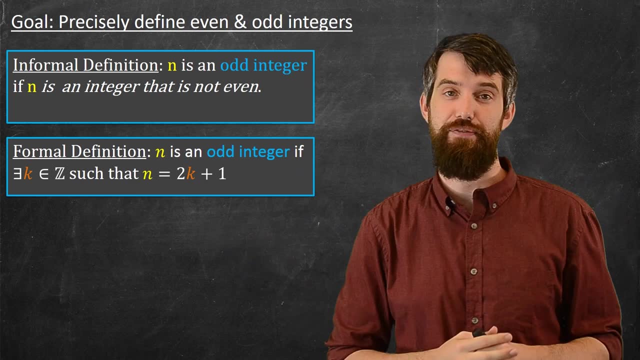 and odd integers. and indeed, in the next video, that's exactly what i'm going to do. i'm going to do our first proof and i'm going to use these definitions of even and odd in the proof that i'm going to do in the next video. you.